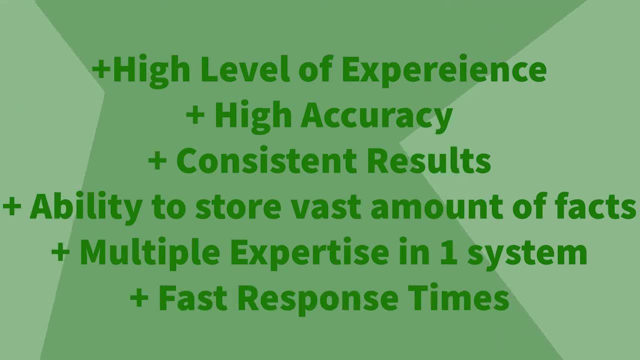 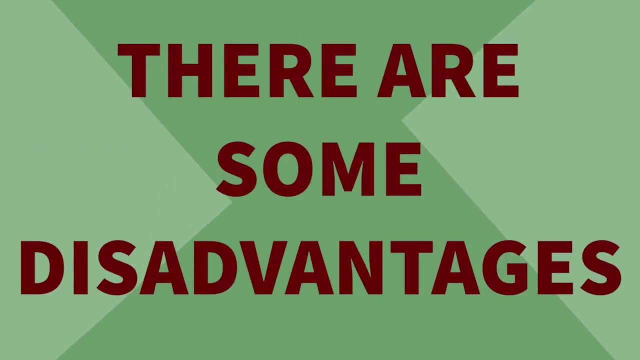 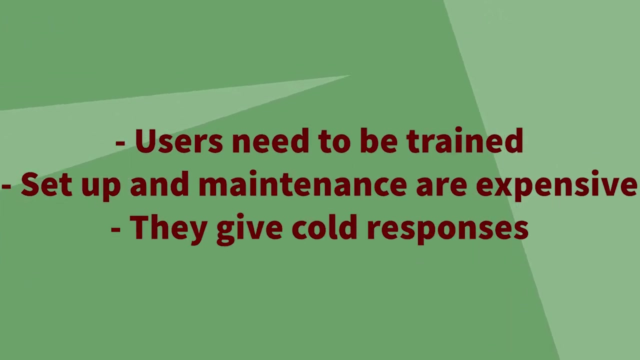 multiple expertise in one system, very fast response times and there are unbiased reportings. However, there are some disadvantages of expert systems, which include: users need to be trained to use expert systems. Setup and maintenance of expert systems are expensive. They give cold responses which may not be appropriate in given circumstances. They're also only as good. 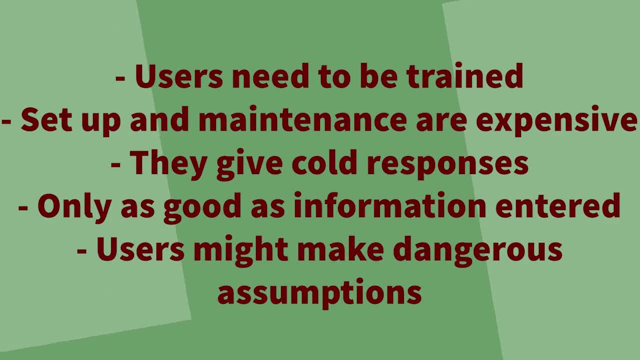 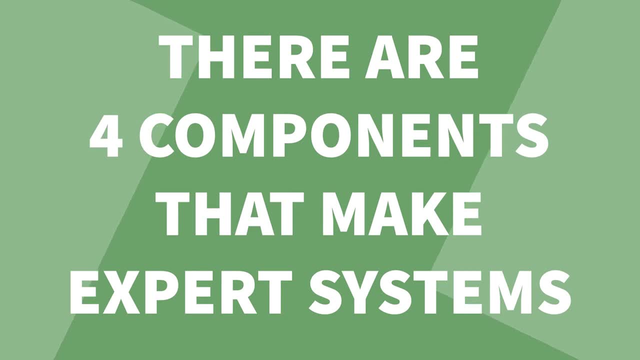 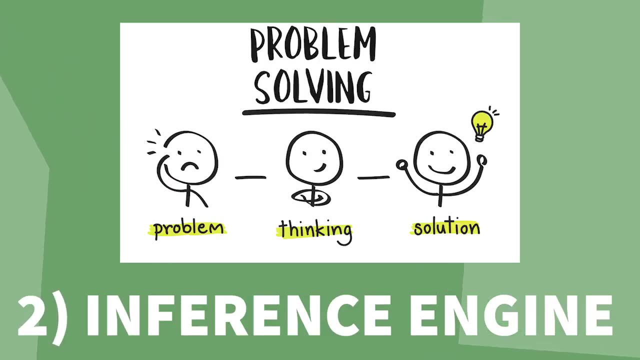 as the information entered. and finally, users might make dangerous assumptions. To finish off, there are four components that make up an expert system. First, you've got the user interface. This is how the expert system interacts with the user. Second, you've got the inference engine. This is: 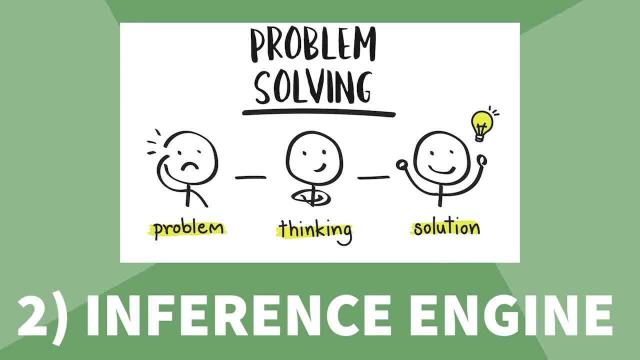 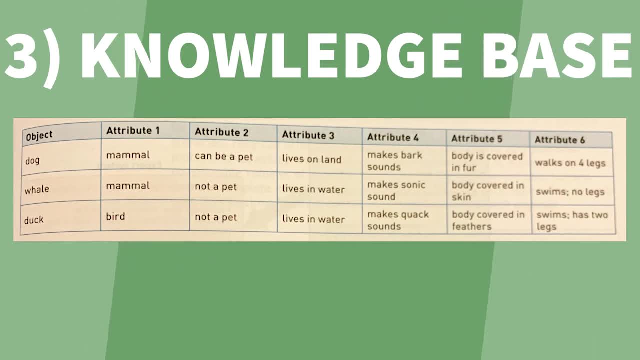 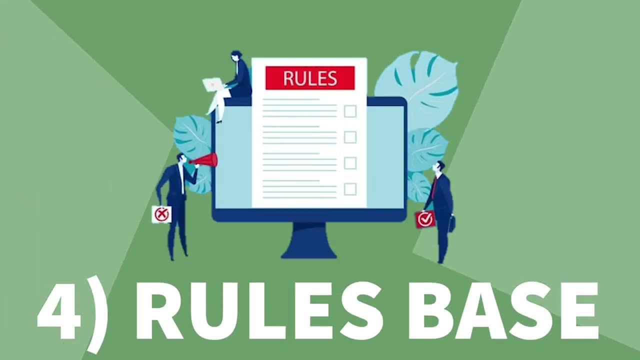 the problem solver. It examines all the knowledge it has to find answers to give to the user. Third is the knowledge base. As the name suggests, this is where all the facts are stored. Here's an example of a knowledge base. and finally, the rules base. The rules base contains rules for the inference engine. 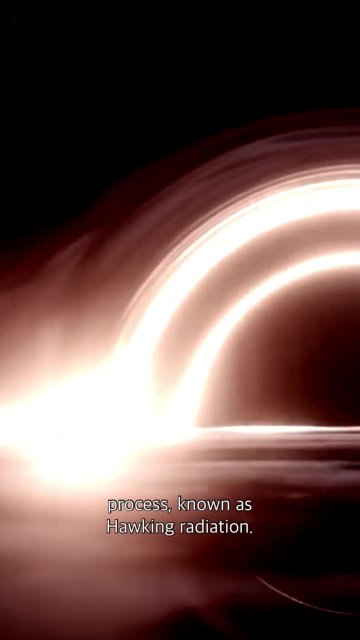 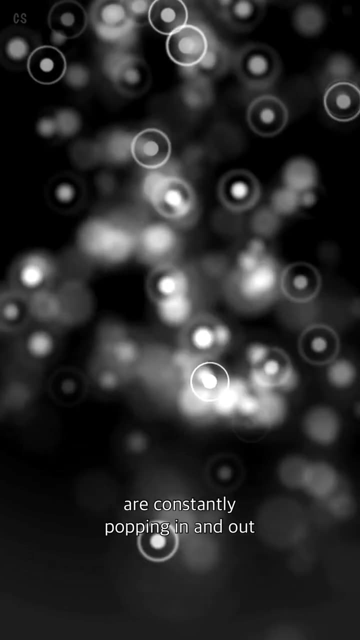 Black holes evaporate due to a theoretical process known as Hawking radiation. According to quantum mechanics and the principles of general relativity, virtual particles are constantly popping in and out of existence in empty space. They usually annihilate each other before they can be detected. 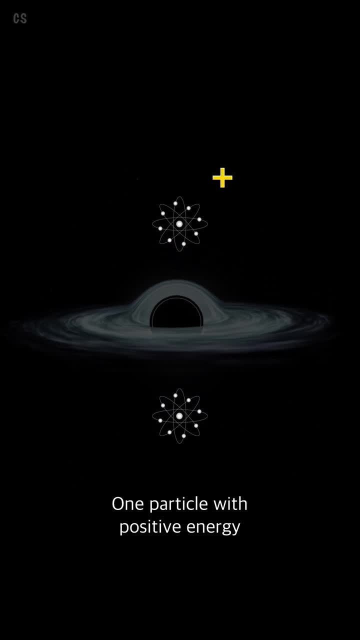 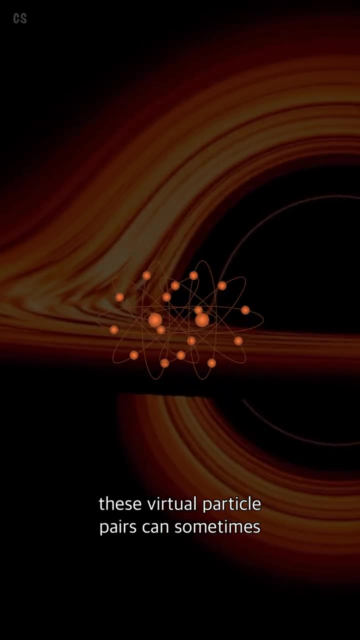 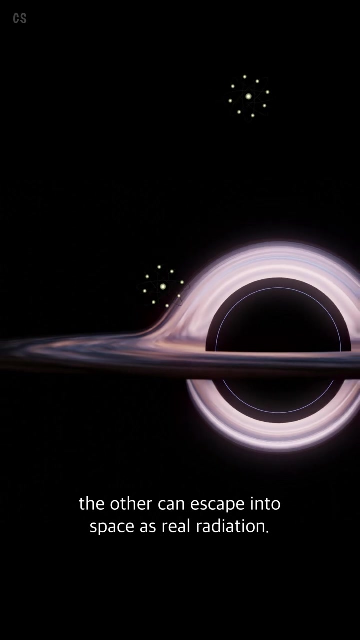 These particles are created in pairs, One particle with positive energy and one with negative energy. Near the event horizon of a black hole, these virtual particle pairs can sometimes be separated. One particle can fall into the black hole, while the other can escape into space as real radiation. The particle that escapes can carry away energy and mass. 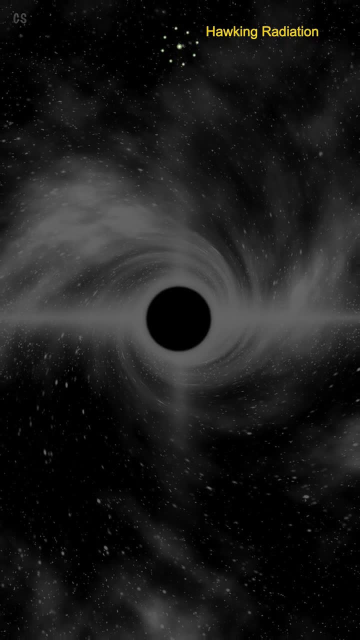 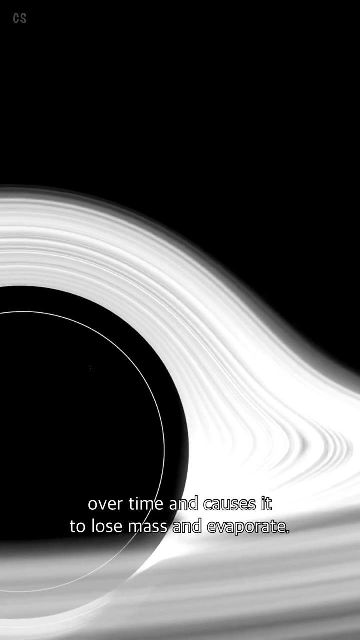 This escaping particle is known as Hawking radiation. Its pair, which falls into black hole, has negative energy or mass, which annihilates the black hole over time and causes it to lose mass and evaporate. 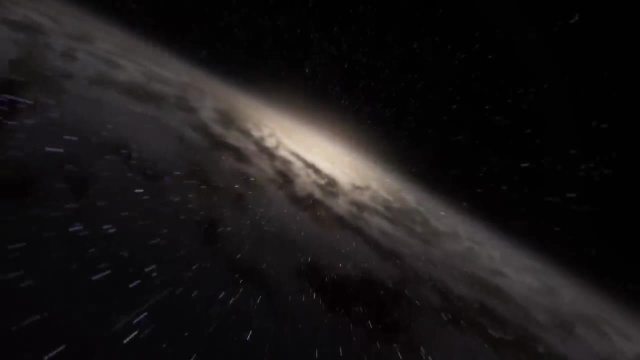 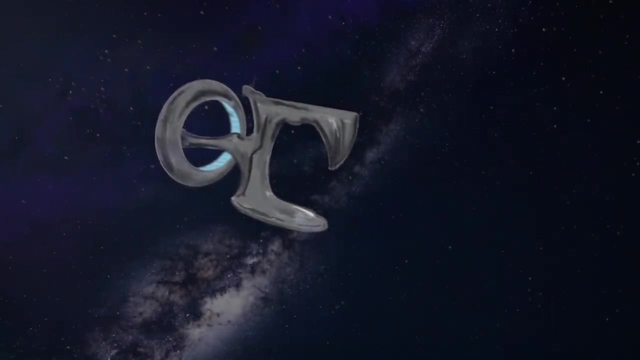 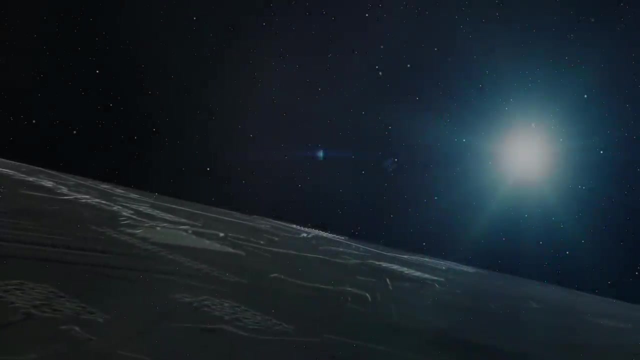 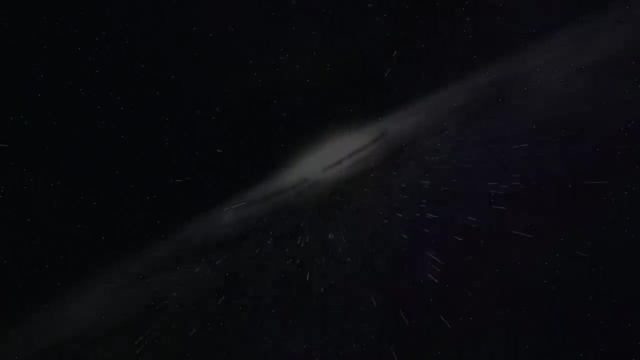 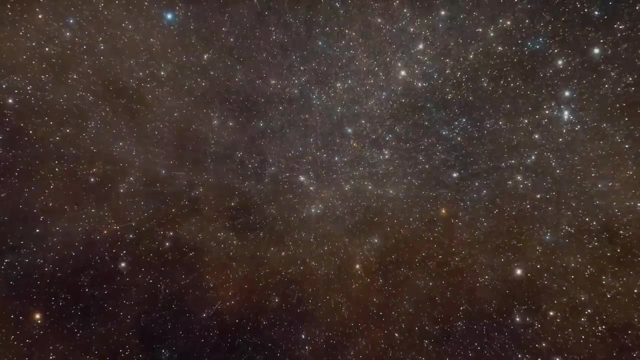 A spacecraft cruises silently through the outer spiral arm of the Milky Way. These voyagers from lands far away aren't in a hurry, Travelling at just 60,000 miles an hour, a crawl by cosmic standards, But they've kept their pace for a million years.